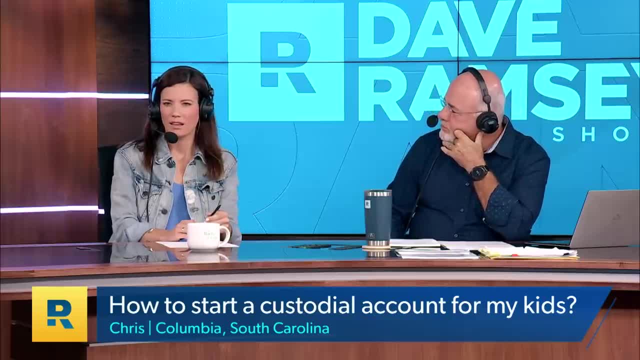 And they just bug me about it. It's not a bugging, but you know they can't. They just ask about it And I figure, if I put it in a brokerage account, that's probably at least a growing interest rate, I guess. 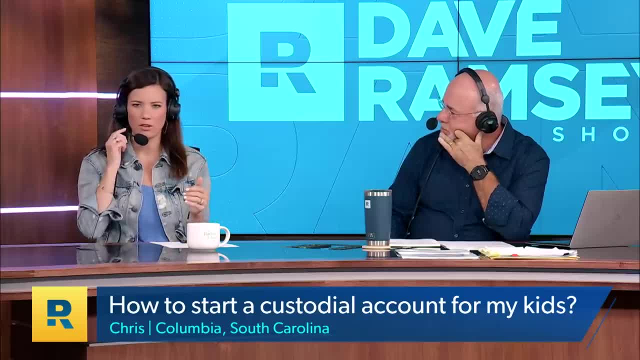 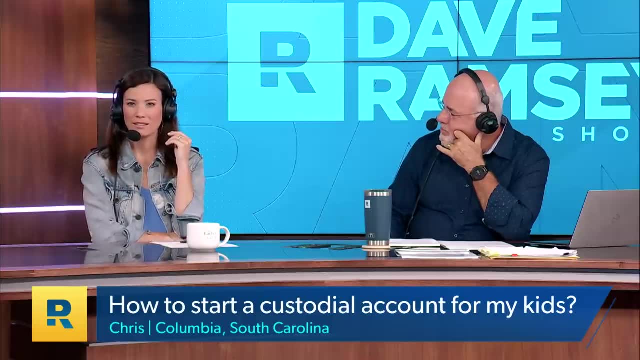 Yeah, but I mean the convenience aspect is what's bothering you, because you're having to go to the bank to get the money out, Where they're 11 and 9, is that what you said? They're 9 and 7.. 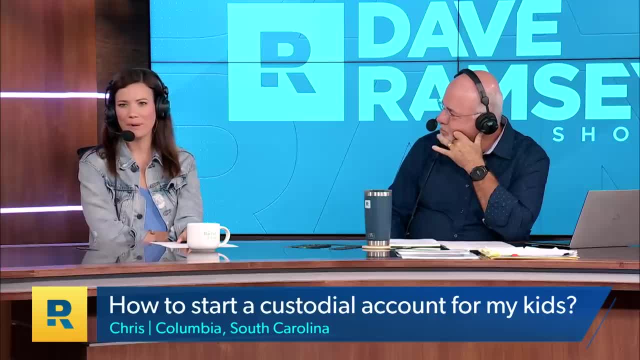 9 and 7,, so even younger. So yeah, I mean at this, this is like basic level teaching kids about money. I mean, all they really need to be doing is giving a little, saving a little, spending a little. 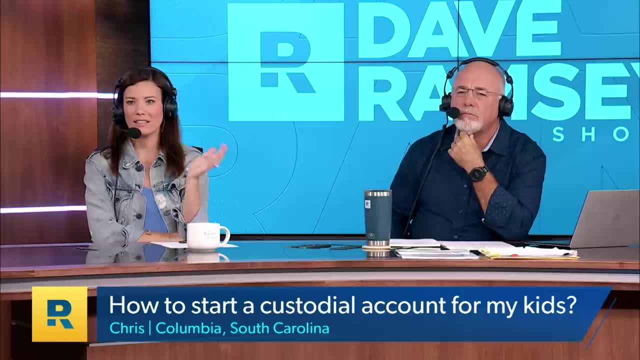 I mean it's not going to be anything insane And so I mean not even having. you could put some of their savings in the bank and it's more long-term for them. Like hey, in the next month or two, if we want to save up and get something. 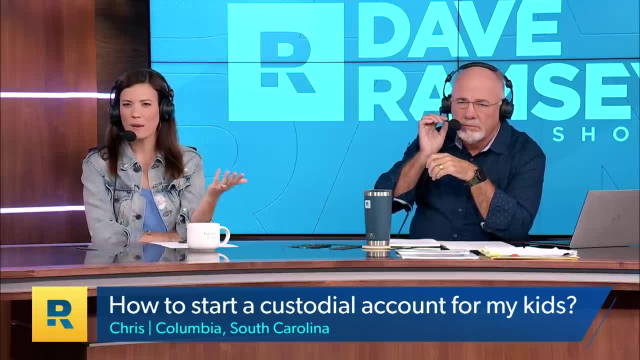 But I would just keep cash at the house at that young of age, depending on how much it is, I mean, if they're getting like big chunks of like birthday money or Christmas money, yeah, you can put it in the account, the savings account. 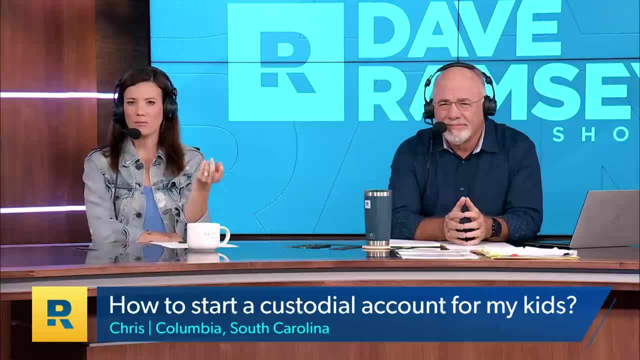 But anything else I would have at home, because, especially for your- you know your, especially your 7-year-old, but your 9-year-old as well- Like when they have cash at home, they feel it We could do the envelopes. 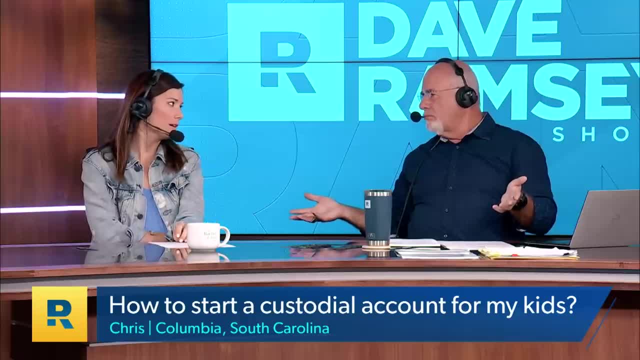 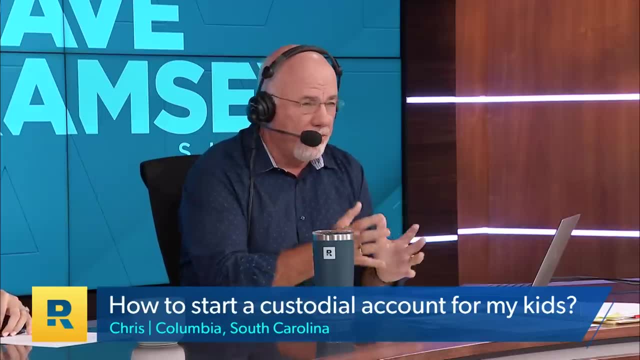 We could have their own envelope, right? Yes, Or the banks is what I was thinking about, Yeah, Yeah. So let's do this. Let us give you the Junior's Adventure Pack, which is the Financial Peace Junior, for teaching kids, little kids, how to handle money. 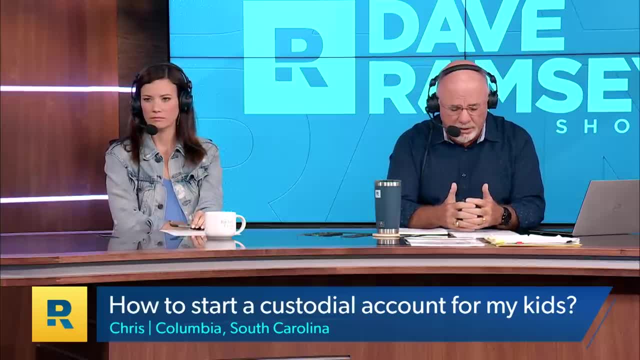 Rachel and I wrote, and we'll also give you a copy of Smart Money, Smart Kids, which is what Rachel and I wrote about parents teaching their kids about money, Because that's really what this question comes down to. okay, Now, what we teach is the kids need to learn four things, and Rachel touched on this. 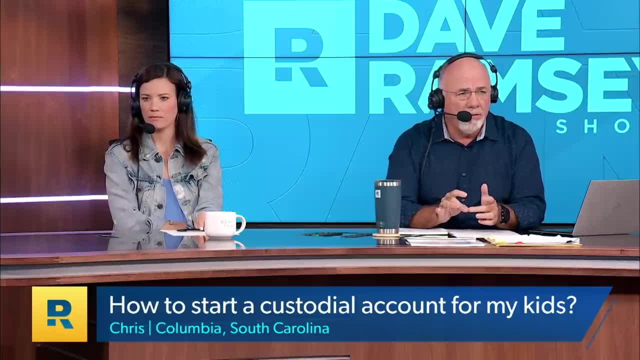 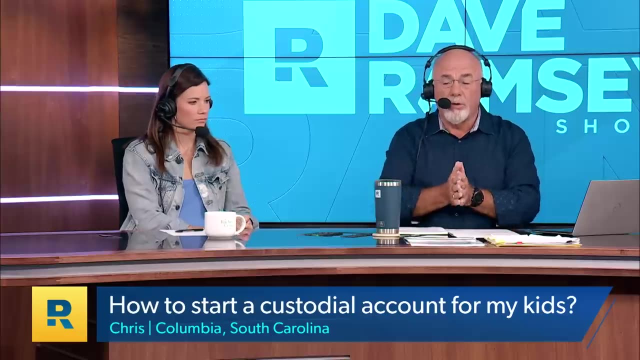 They need to learn to work, which is where money comes from. They need to learn to give, They need to learn to spend wisely, under the parent's direction, and, of course, to save. And so the difference is, instead of opening a brokerage account to keep them from bugging you, I will put them on a system that says: 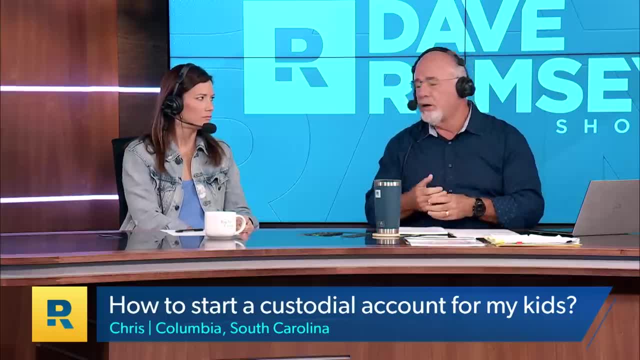 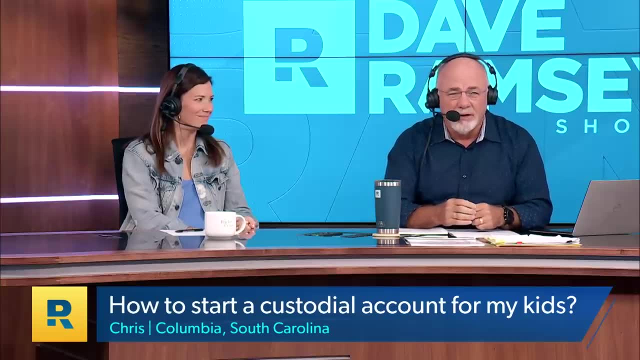 kids. my job is to help you, as your dad, learn how to handle money. so when you're old, you're not one of those old broke people, Okay, Like all our freaking friends, right? So you know, and so then they get. 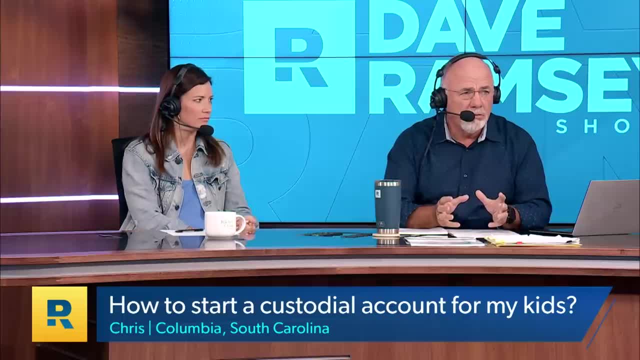 When our kids would earn some money- end quotes- for doing a chore like feeding the dog or something really difficult like that which you hardly break a sweat doing right, But they would earn money for doing a chore, then we would divide the chore money. we call it commissions. 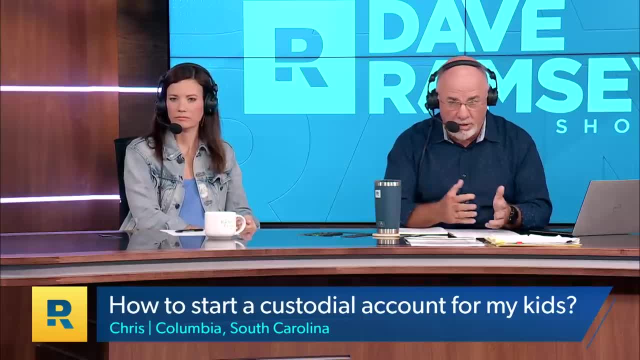 You're not on allowance, you're on commissions, You're not, You work, you get paid, You don't work, you don't get paid. Then we would divide that up into those three envelopes, And the kit I'm going to send you has three envelopes. 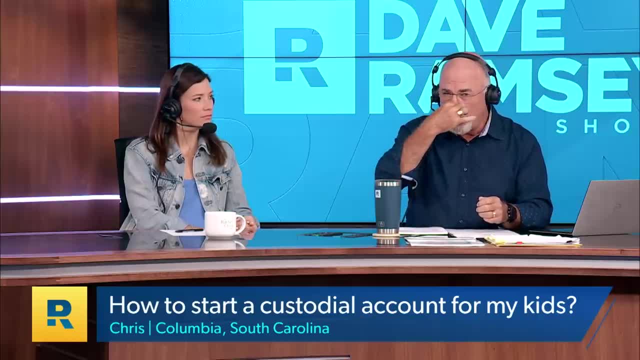 It has a giving envelope, a saving envelope and a spending envelope And so if they get, If they get ready to say I want to spend some money, do you have it in your spending envelope? Because we put some in there from when you worked. 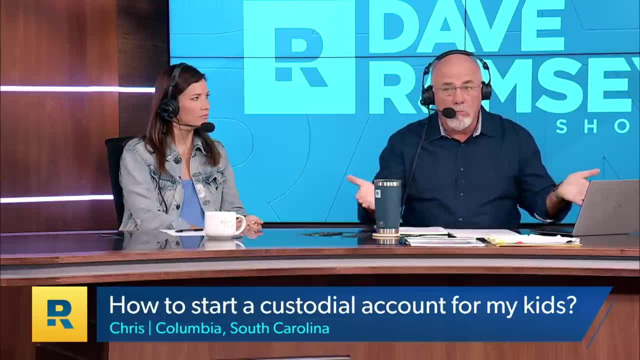 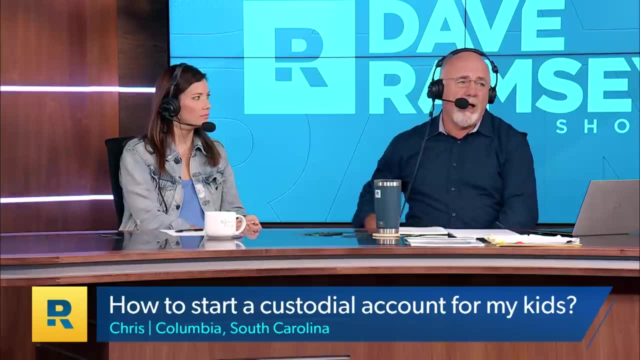 And then you can have the discussion of: oh, there's not enough money, Well, you're going to have to wait and work some more. Or you can have the discussion of: you can buy that cheap one if you want to buy it, but it'll be broken by Friday. 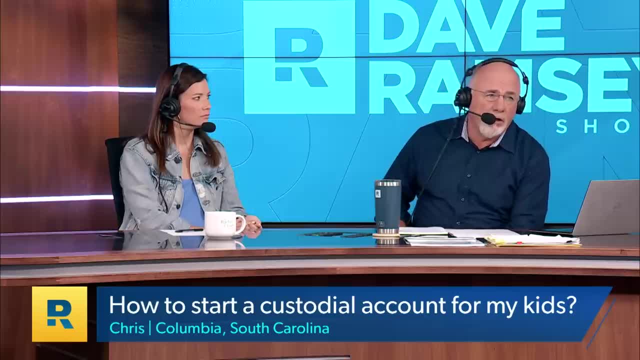 Or you can wait a little bit and buy a good one that will last you and you can pass it down to your grandkids. And we had lots of value discussions about purchases. Rachel generally just bought it. Daniel was very purposeful and goal-driven about his purchases. 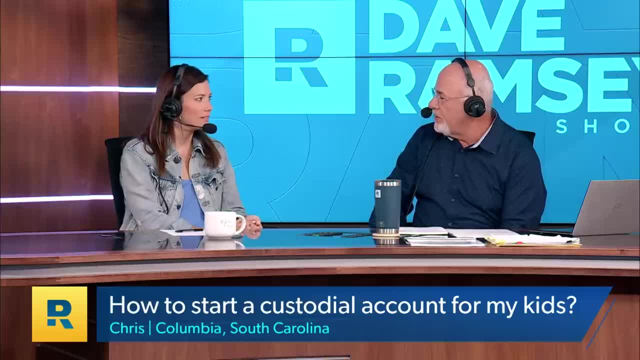 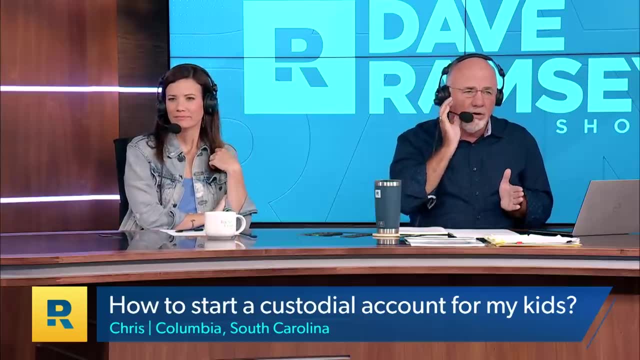 And Denise was what compliant I don't know Didn't even spend money. Yeah, she didn't spend money. She's a saver, But you need to make kids, coach kids in all four areas. Not working is not an option. 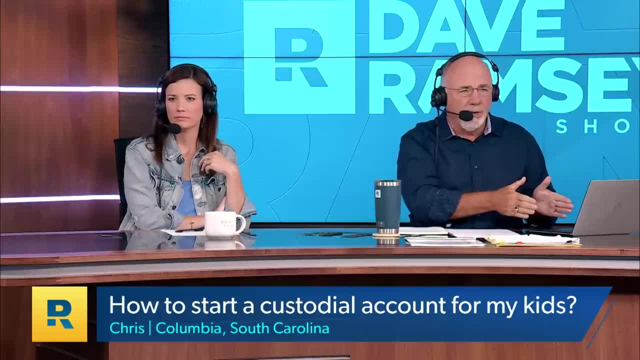 Not being generous is not an option. Not saving is not an option. Not spending money wisely is not an option. So you can't be only saving. Or sometimes, sweet little kids, they want to give all their money away. Well no, I don't want to teach you that way. 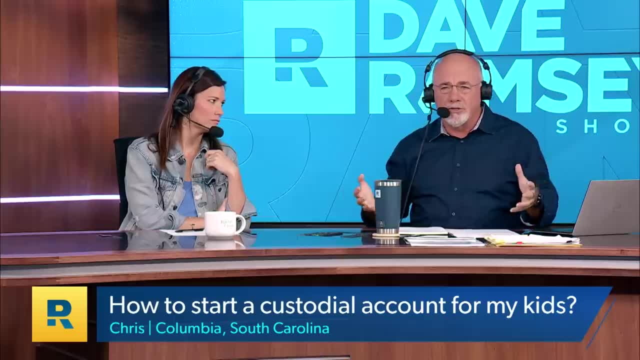 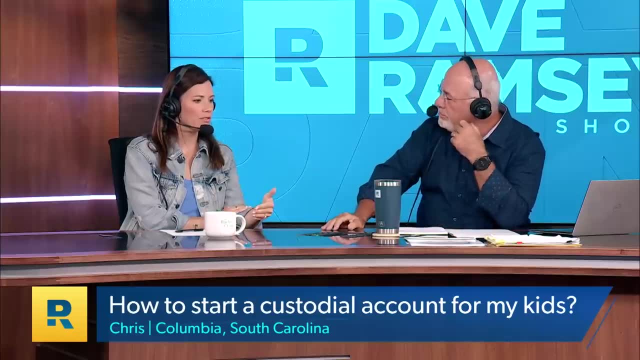 I want to encourage you in your generosity, your outlandish generosity, But you always should have some saved and you should always have some to spend as well. Yeah, because I mean, as an adult, primarily those are the three things you do with money. 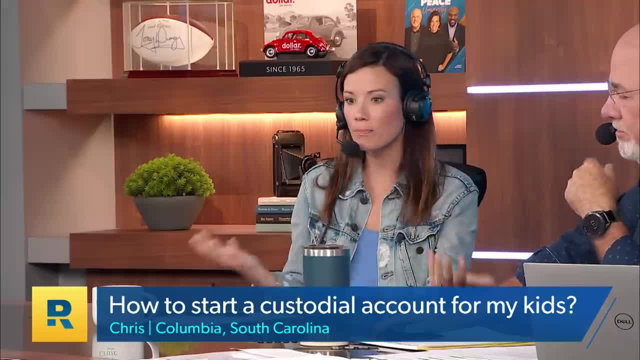 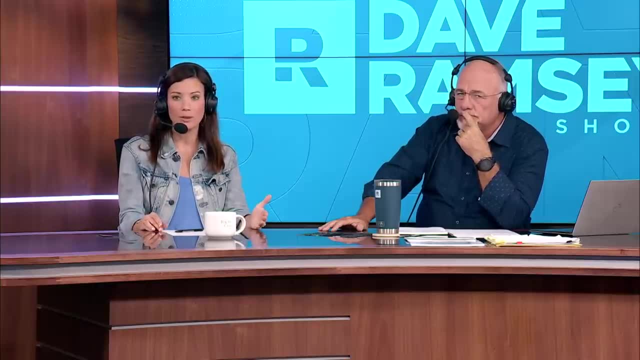 I mean, obviously your saving can be more complicated and investing and all that, But basically that's what you do with money: You give, save and spend, And so teaching those boundaries is huge. And then I mean: and Chris, if they're not doing like just work around the house? 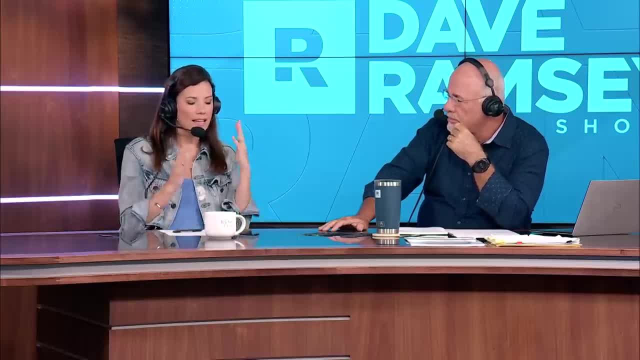 simple stuff: earning that money. I mean it's, and again, it's, very age-appropriate, But, man, the award is amazing, Amelia, I didn't even tell you this, Papa Dave, you'll be so proud. 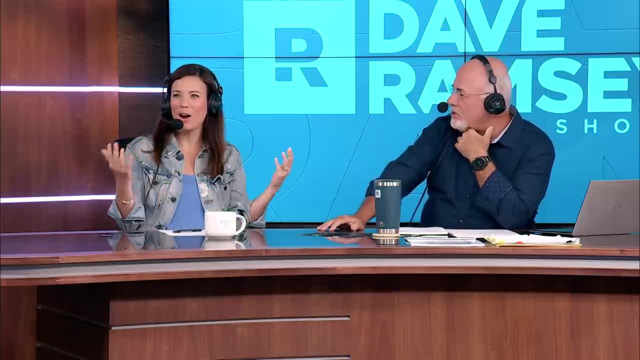 Okay, I'm ready. She did some chores, She what. She did some chores. What did she do? She actually swept the kitchen. I didn't even ask her to, But she was like Mom, can I sweep to earn a dollar? 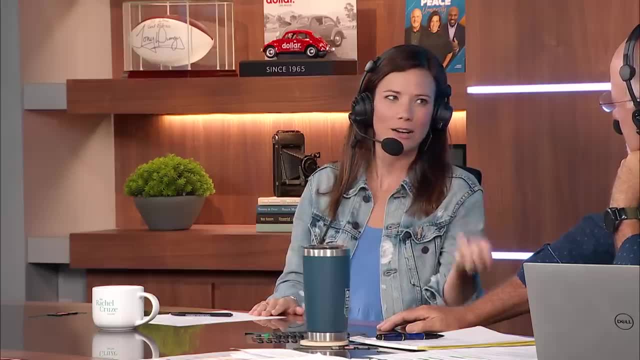 I was like sure, let's just do it, Because we have like ten bucks and ones in our like little junk drawer, So that's what I like. gave it to her. So she did that- Carried plates to the sink. 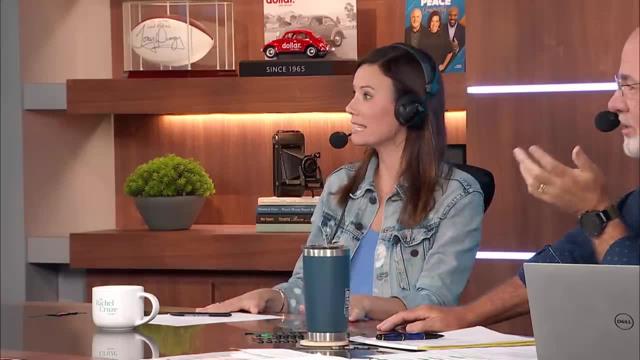 I mean, she just turned it on, She just turned five, So it's like it's low-ball stuff. Well, you don't send a five-year-old to the salt mines, No, so you do. So we did six and we went on Amazon. 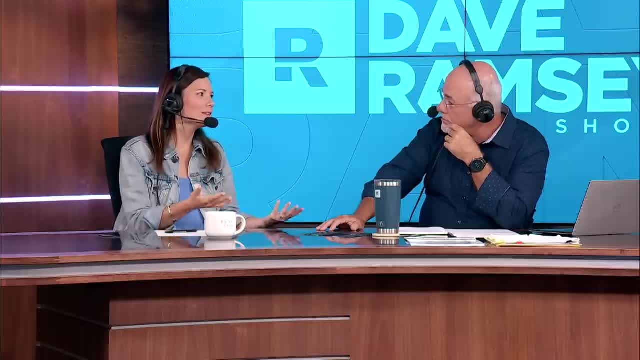 She bought a Polly Pocket for $6.99.. I paid the tax. I was like you know what I'm going to be a graceful mother and just your five. So I was like I'll pay the tax because she saw the six on Amazon. 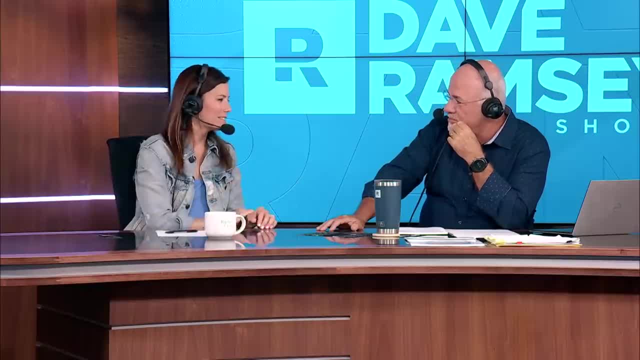 She was like: it's six, Mom, it's six and I have $6.. And I was like, yeah, you're great, Yes, that's great. But then she got very confused that the money was still there even though the Polly Pocket arrived. 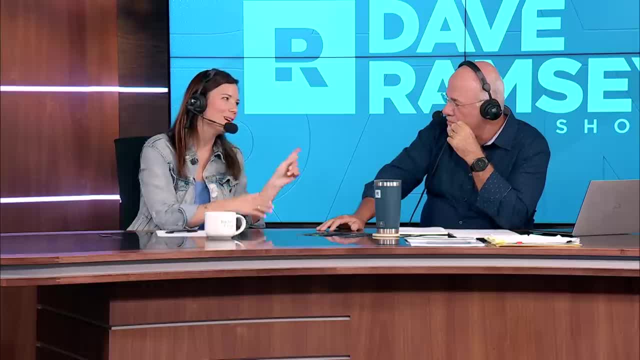 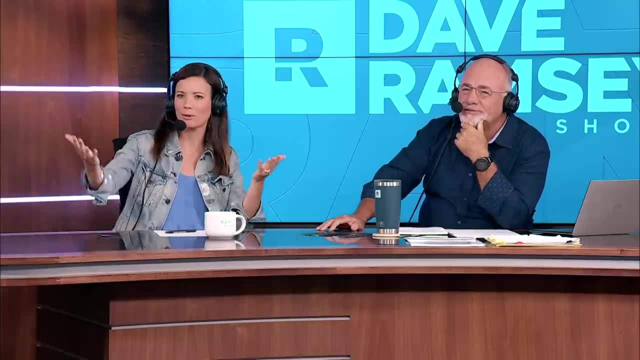 But I took her money And so the whole process of buying online is very complicated for kids. They don't quite understand it, So it probably would have been a little bit more beneficial to like, put on the masks and go to Target and buy. 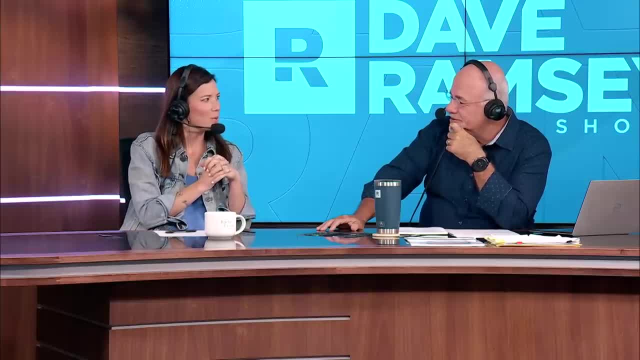 But I was a little too lazy So I was like we're just going to Amazon it and have to walk through. But hey, that's a modern day. Still, you did it. No, You did it because what most parents do is nothing. 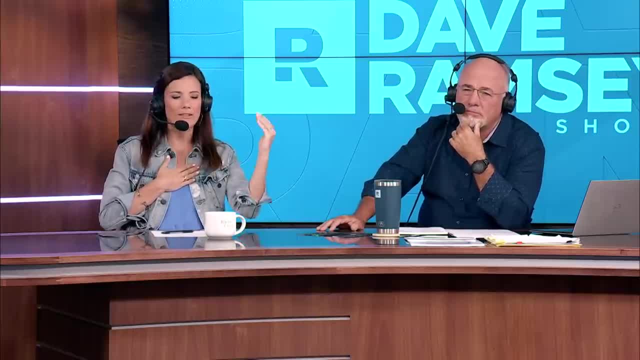 Well, and the story wasn't about me doing it, But what I was going to say is the effects of what happened. she made me like take a video of her to send it to a girl that babysits for us, because she was like: tell Maggie. 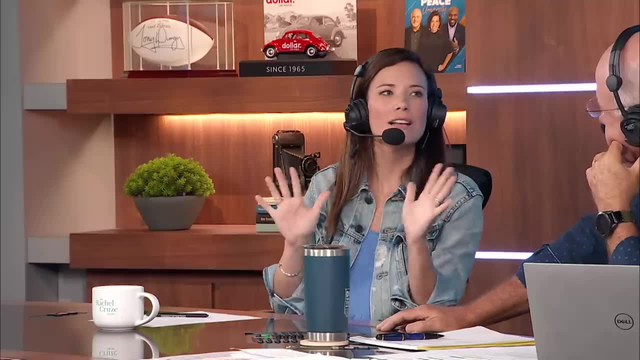 Then I bought my own Polly Pocket. I was like, okay, so we did it, Like she was, oh, it was just, it was amazing, She just could not. I mean talked about it for three days. So anyways, it works. 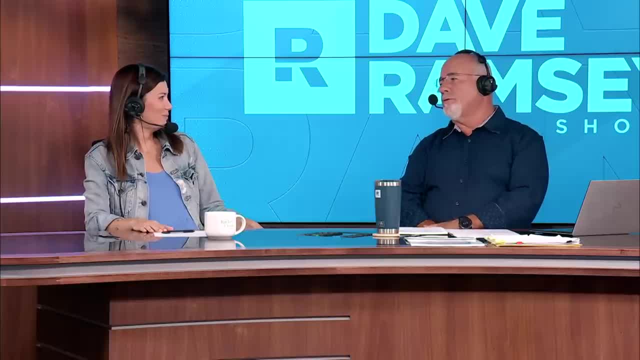 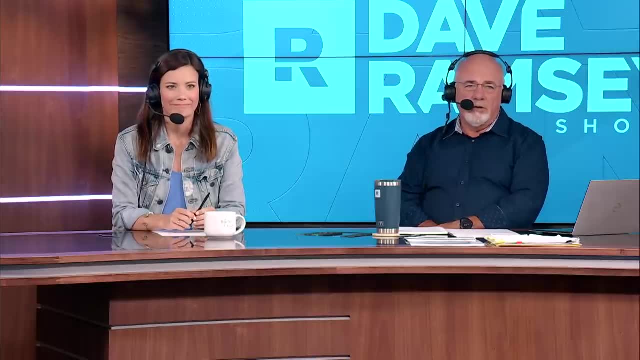 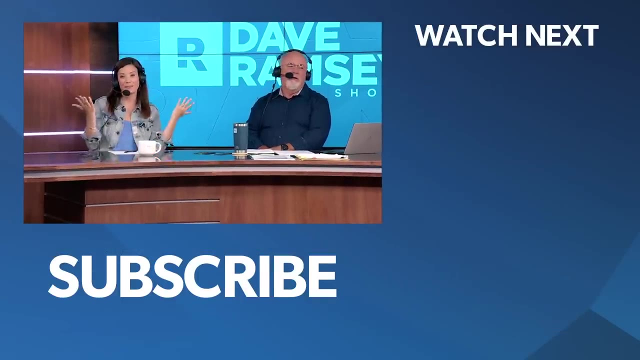 It gives anyone who works and earns gains dignity as well as money. It's true, Not working does not give you dignity, And so it's good that Amelia's sweeping the kitchen. She actually did pretty good, Hey, I bet, I bet.